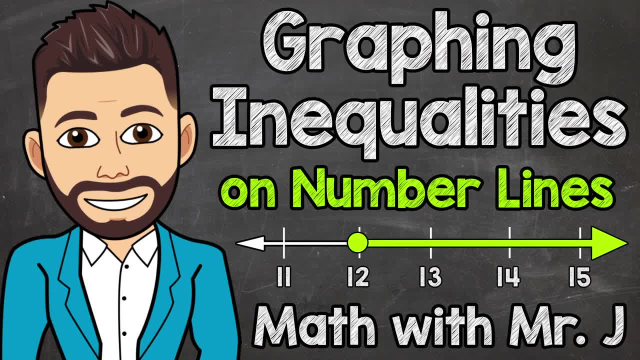 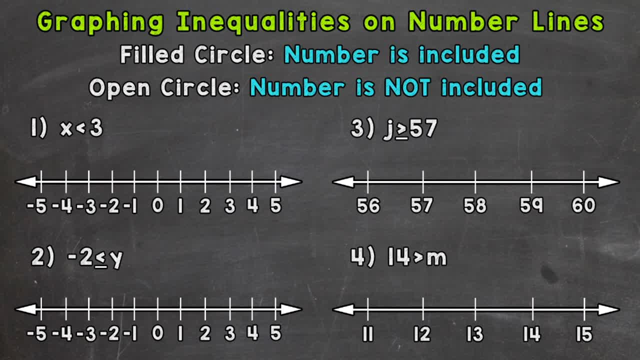 Welcome to Math with Mr J. In this video I'm going to cover how to graph inequalities on number lines. Now, when we graph inequalities on number lines, this really helps us visualize what inequalities mean and gives us a better overall understanding of inequalities. We'll go through four examples together here. 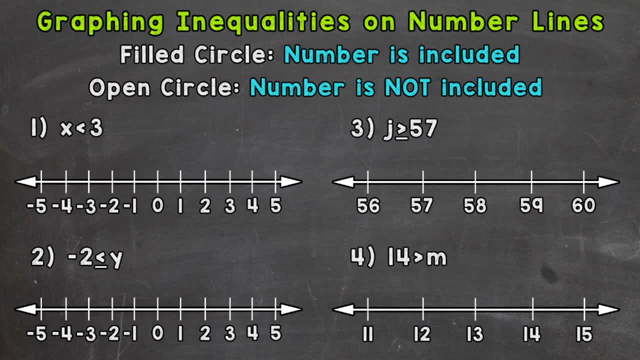 in order to get this down Now, at the top of the screen there are two very important notes that will help us with graphing these inequalities on number lines. So if we use a filled circle, the number is included. If we use an open circle, the number is not included, And you'll see exactly. 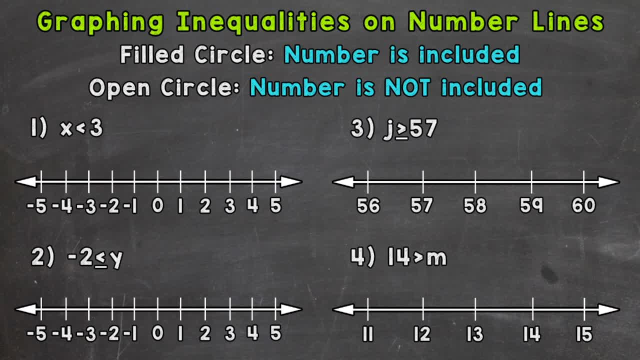 what that means as we go through our examples. So let's jump into number one, where we have: x is less than three. So our variable x here has to have a value less than three. Now, this is not a less than or equal to symbol. 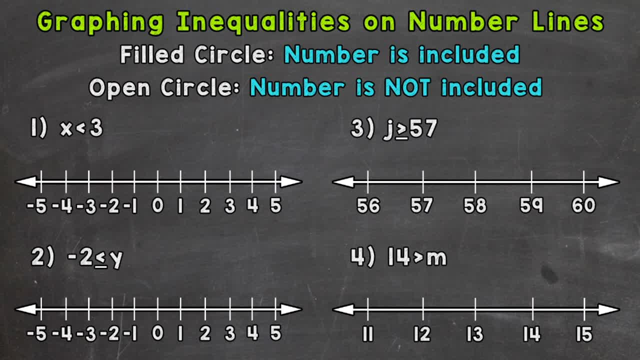 so we want an open circle because three is not included. So we're going to put an open circle on three and again that indicates that we are not including three in our solutions. Now x is less than three, so any number less than three is going to be. 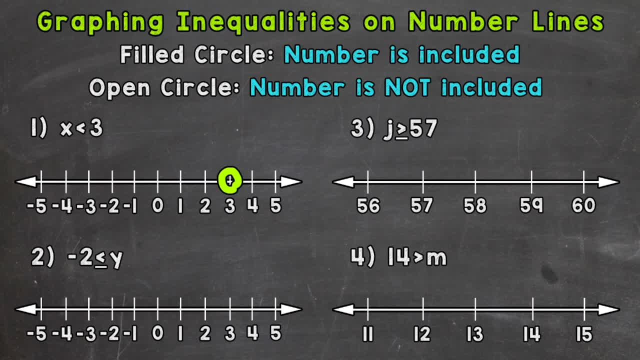 solution. So we draw an arrow pointing in the direction of the numbers less than 3.. This is going to represent all of the solutions that will work for this inequality. So let's draw an arrow to the left here and include all of the values less than 3.. So, for example, if we were to say: 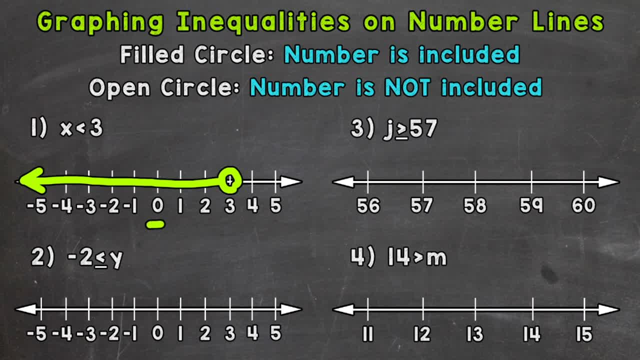 x equals 0, right here, x equals 0, 0 is less than 3.. That would be a solution. So on and so forth, for all of those values less than 3.. We have an infinite amount of solutions, and that's what that. 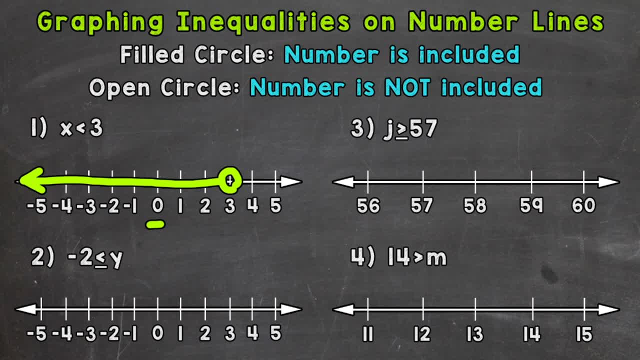 arrow represents. And again we used an open circle because 3 is not included in our solutions. So let's move on to number 2, where we have negative 2 is less than or equal to y. So for number 2, anything greater than or equal to negative 2 would be a solution. So what we can. 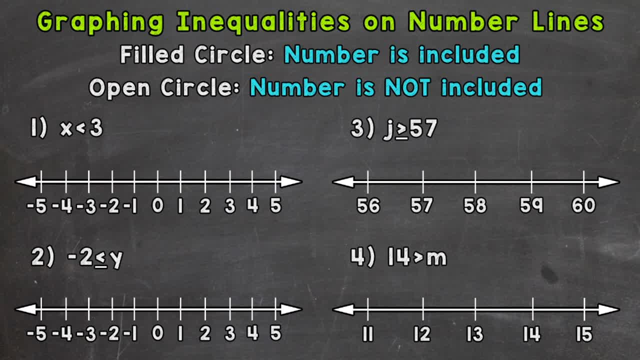 what that means as we go through our examples. So let's jump into number one, where we have: x is less than three. So our variable x here has to have a value less than three. Now, this is not a less than or equal to symbol. 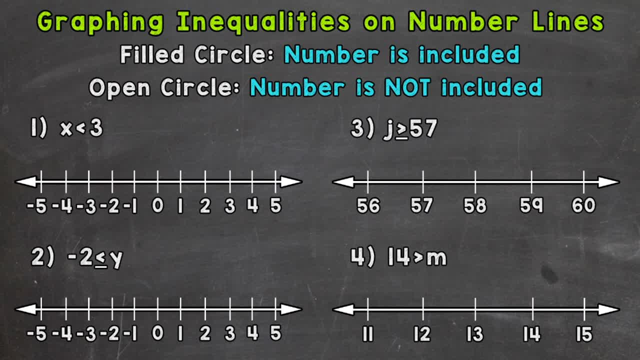 We want an open circle because three is not included. So we're going to put an open circle on three And again that indicates that we are not including three in our solutions. Now x is less than three, So any number less than three is going to be. 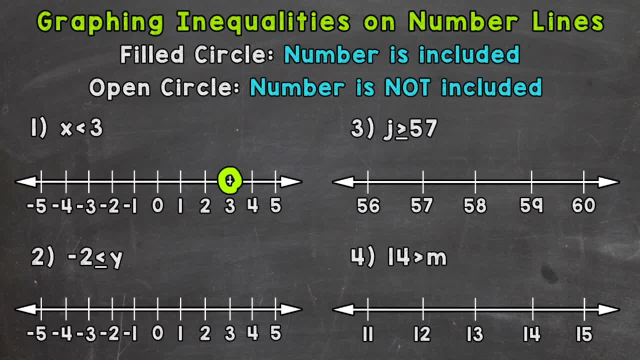 aurob or갈3ol3.. Now how to graph inequalities on 3D. Firstly, we have x. here has to have a value, correct solution. So we draw an arrow pointing in the direction of the numbers less than three. This is going to represent all of the solutions that will work for this inequality, So let's draw. 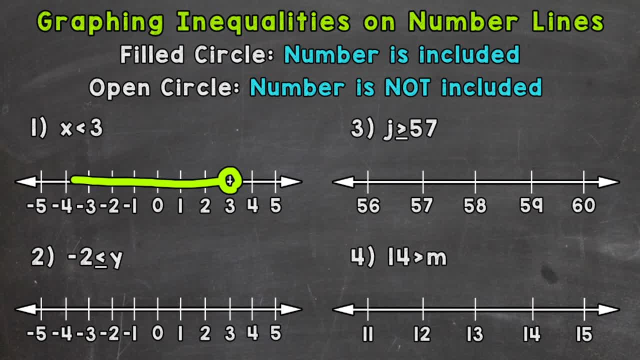 an arrow to the left here and include all of the values less than three. So, for example, if we were to say x equals zero, right here, x equals zero, zero is less than three, that would be a solution. so on and so forth, For all of those values less than three, we have an infinite amount of solutions. 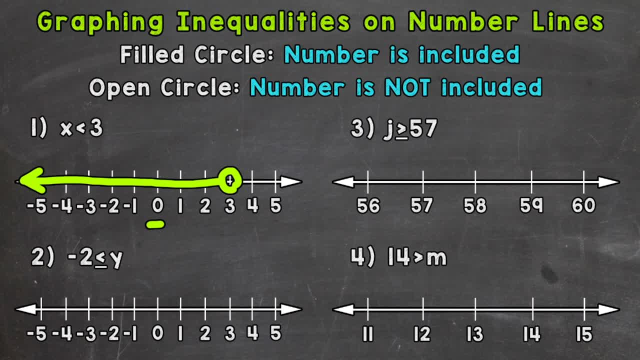 And that's what that arrow represents. And again, we used an open circle because three is not included in our solutions. So let's move on to number two, where we have negative two is less than or equal. So for number two, anything greater than or equal to negative two would be a solution. So what we 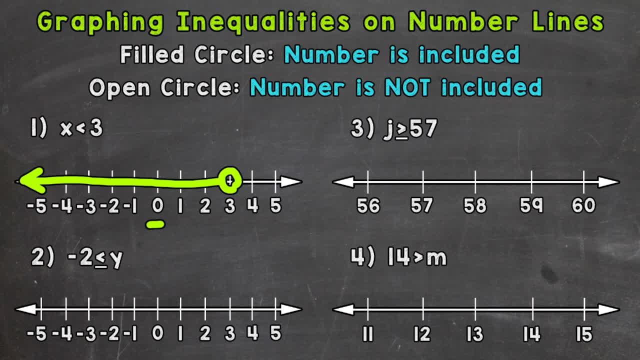 can do. let's start at negative two, And this is a filled circle because negative two is included, because we have an or equal to symbol. So let's fill in our circle here Now. y can be anything greater than, or equal to, negative two, So we want all the values that are greater than this. 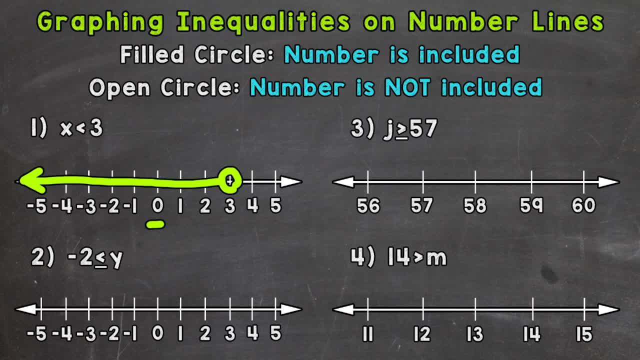 do. let's start at negative 2.. And this is a filled circle because negative 2 is included, because we have an or equal to symbol. So let's fill in our circle here Now. y can be anything greater than, or equal to, negative 2.. So we want all the values that are greater than this to be: 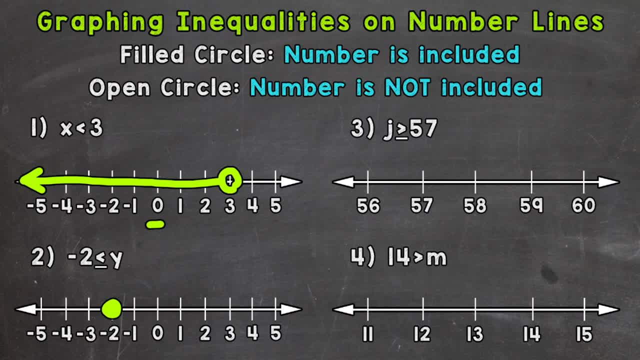 represented. So we need our arrow pointing to the right here. And that indicates everything greater than negative 2 is going to be a solution. So, for example, let's just pick out 4.. And if we were to plug in 4, negative 2 is less than or equal to 4.. Well, that would be a solution. That would 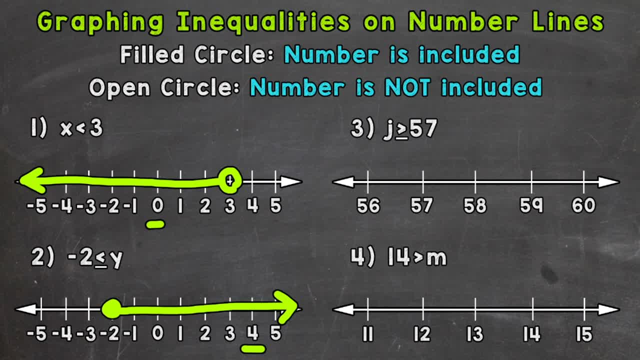 be correct. So that arrow represents all of the numbers greater than negative 2.. And then our arrow here represents negative 2 being included in our solutions because again we had an or equal to symbol On to number 3, where we have j is greater than or equal to 57.. So this is another. 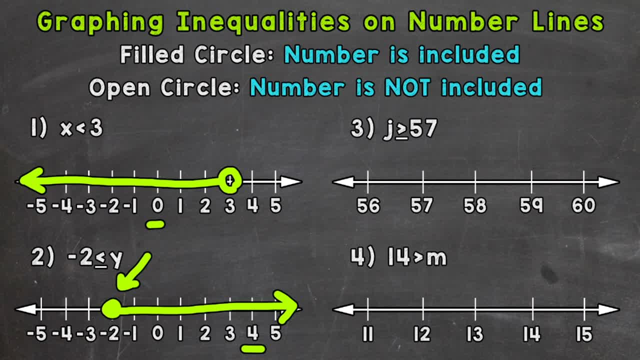 one that we have or equal to. So j any value greater than or equal to 57 would be a solution. So we need a filled circle including 57. And then we want all the values that are greater than 57 to be represented, And that's going. 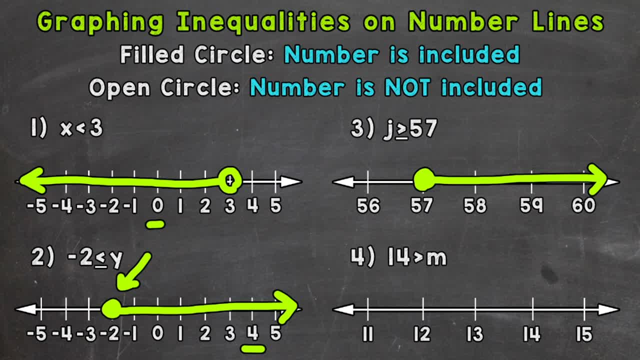 to be our arrow here. So, for example, 60 would be a solution. 60 is greater than or equal to 57.. So the arrow represents all values greater than 57.. And the filled circle represents 57 being included in our solutions. 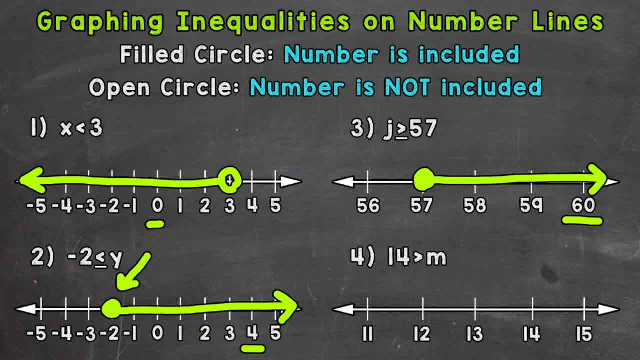 So let's move on to number 4, where we have: 14 is greater than m. So 14 is not included in the solutions here, because we do not have an or equal to symbol, We just have a greater than symbol. So we're going to use an open circle because we do not want to include 14.. Now, correct solutions. 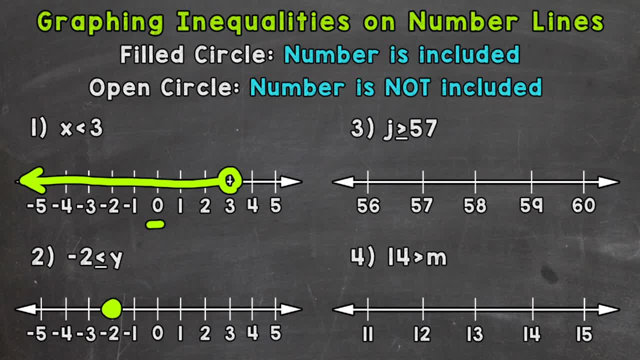 to be equal to negative two. So we want all the values that are greater than this to be represented. So we need our arrow pointing to the right here And that indicates everything greater than negative two is going to be a solution. So, for example, let's just pick out four, And if we 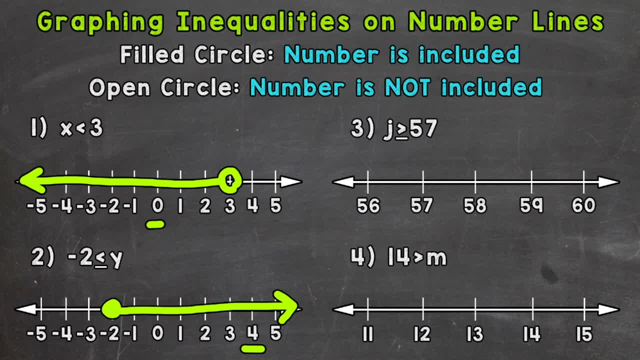 were to plug in four: negative two is less than or equal to four. well, that would be a solution. that would be correct. So that arrow represents all of the numbers greater than negative two, and then our filled circle. So that would be a solution. So let's pick out four. and if we were to 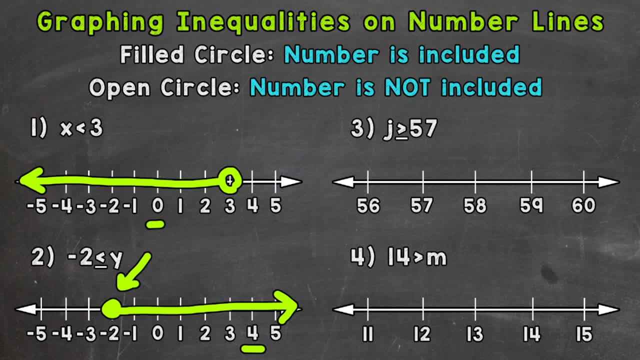 circle right here represents negative two being included in our solutions because again we had an or equal to symbol. On to number three, where we have j is greater than or equal to 57. So this is another one that we have or equal to So j: any value greater than or equal to 57. 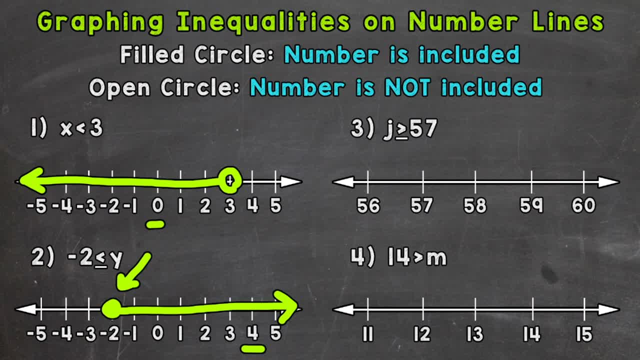 would be a solution. So we need a filled circle including 57.. Then we want all the values that are greater than 57 to be represented, And that's going to be our arrow here. So, for example, 60 would be a solution. 60 is greater than or equal to 57.. 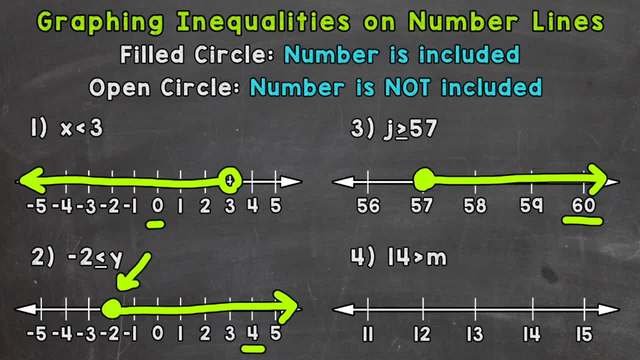 So the arrow represents all values greater than 57.. And the filled circle represents 67 being included in our solutions. And then we want all the values that are greater than or equal to 57 to be represented. So that's the arrow here. And then we want all the values that are greater than or equal to. 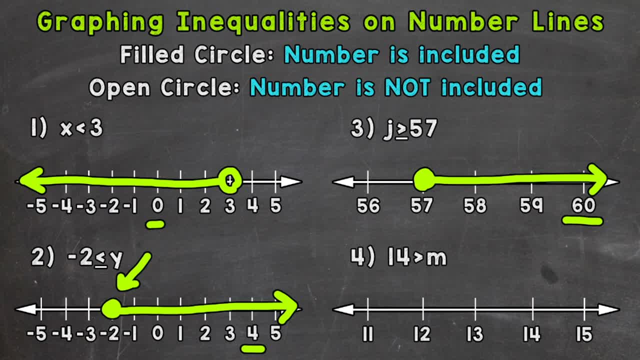 our solutions. So let's move on to number four, where we have 14 is greater than M. So 14 is not included in the solutions here, because we do not have an or equal to symbol. we just have a greater than symbol. So we're going to use an open. 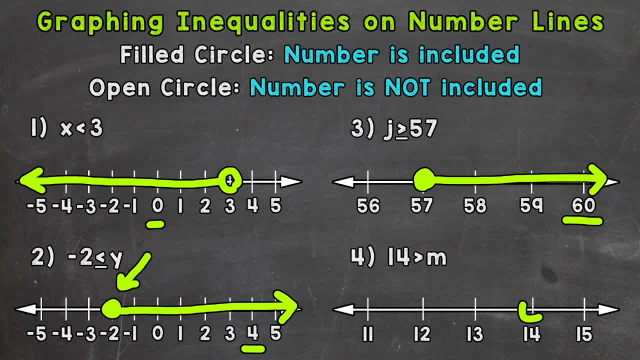 circle because we do not want to include 14.. Now, correct solutions are going to be any numbers less than 14.. So we're going to represent that with an arrow pointing in the direction of all the numbers less than 14.. So, for example, if we were to say: 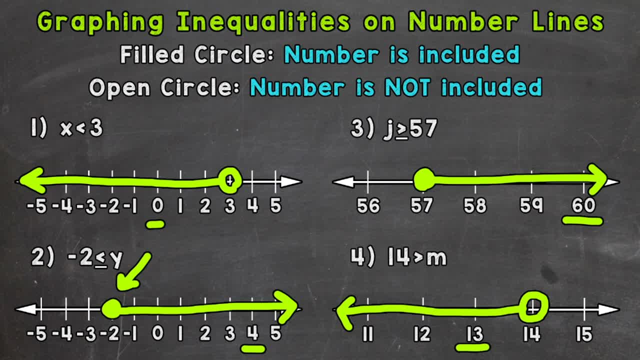 that M equals 13. would that be a correct solution? Well, 14 is greater than 13.. Yes, that is correct, and we have an infinite amount of solutions, so that arrow represents all of those solutions that are less than 14. and again, an open.